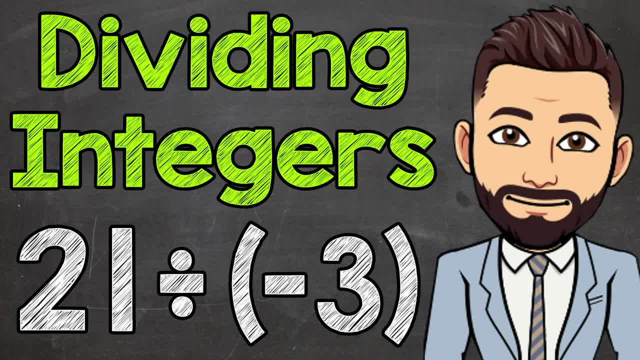 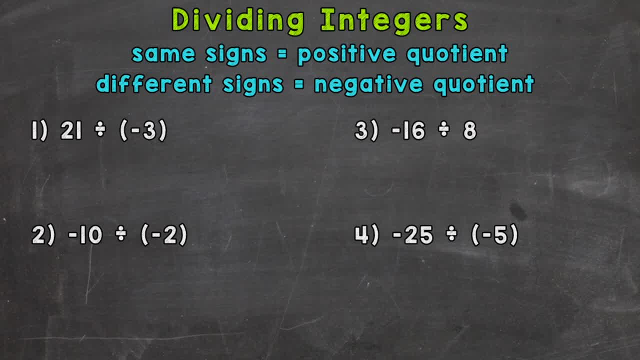 Welcome to Math with Mr J. In this video, I'm going to cover how to divide integers. Now we're going to be incorporating both negative and positive integers in the four examples that we're going to go through together in order to get this down. 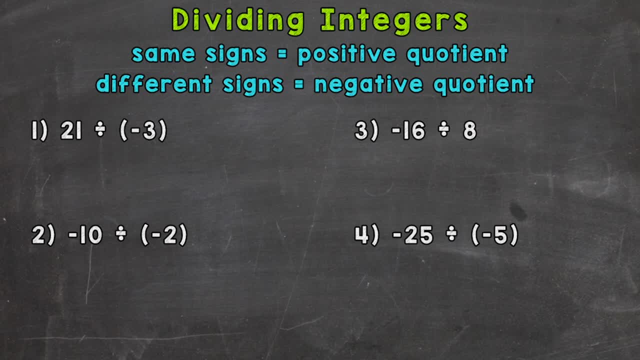 So let's jump right into number one, where we have 21 divided by negative 3.. Now, at the top of the screen, we have some very important information about how to solve these. So if we have the same signs, so a positive divided by a positive- 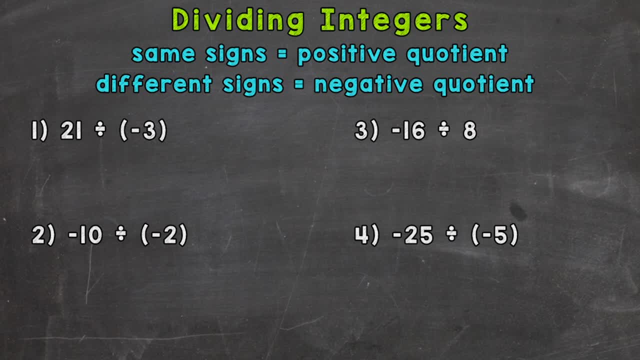 or a negative divided by a negative, we will get a positive quotient. If you have different signs, so a positive divided by a negative or a negative divided by a positive, then we end up with a negative quotient. So let's do 21 divided by negative, 3 here. 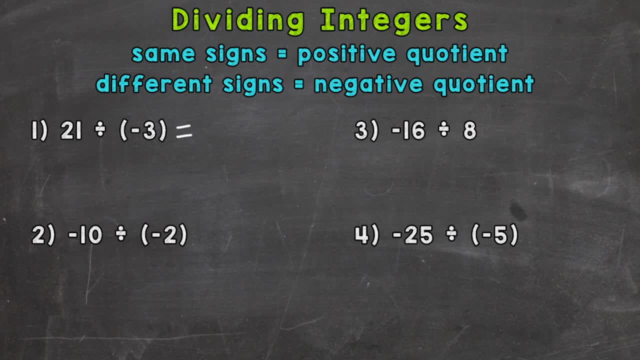 And we can just think of it as the division fact 21 divided by 3. So that gives us 7.. Now, in the case of number 1, we have a positive divided by a negative, So we have different signs. So that is going to give us a negative quotient. 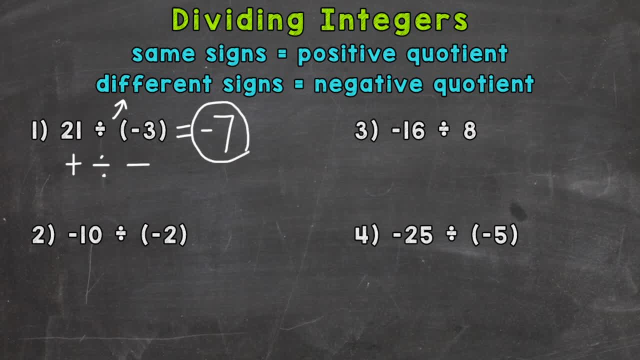 So our final answer is negative 7.. On to number 2, where we have negative 10 divided by negative 2. Let's just think of this as 10 divided by 2. Which gives us 5. Now we have a negative divided by a negative. 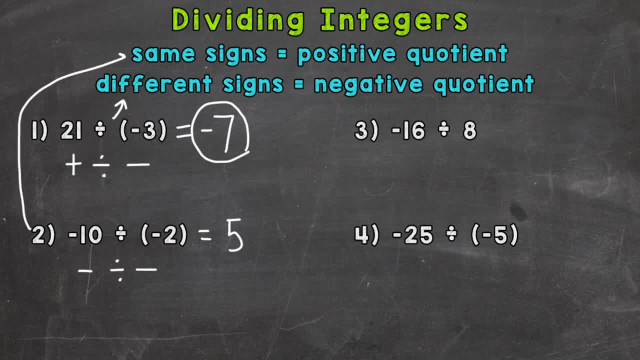 So number 2 would be same signs, right, Negative and negative. That's going to give us a positive quotient, So our final answer is a positive 5.. Number 3, we have negative 16 divided by 8.. So again, we can think of this as just the fact. 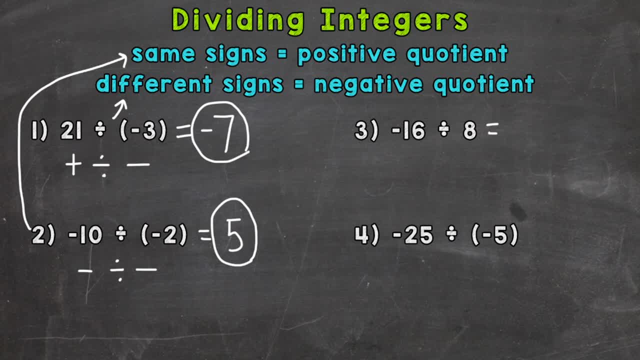 16 divided by 8. Which gives us? Which gives us 2.. Let's look at our signs. So we have negative divided by a positive. So different signs equals negative quotient. So our quotient or final answer: there is going to be a negative 2.. 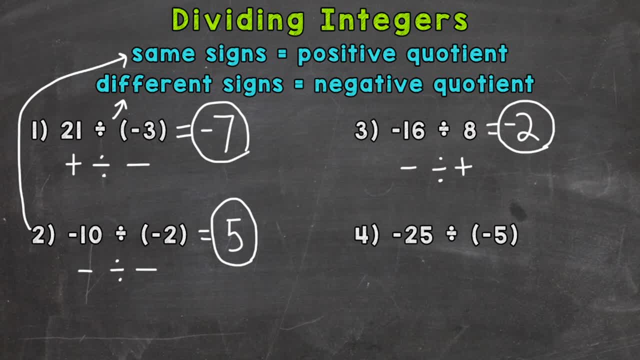 And lastly, number 4, we have a negative divided by a negative. So negative 25 divided by negative, 5.. So 25 divided by 5 is going to give us 5.. Now let's determine If that's going to be a positive quotient or a negative quotient.